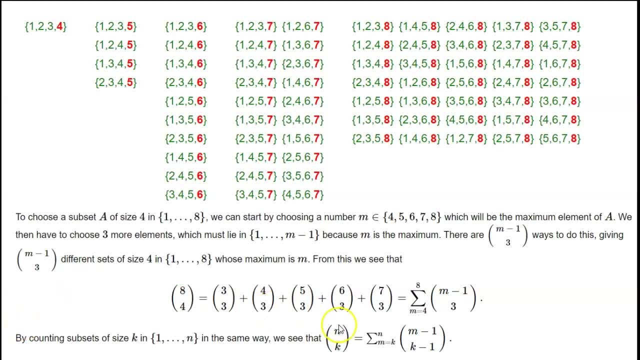 So this demonstration explains the proof of this identity that we've written down at the bottom here. that n choose k is the sum from m is k all the way up to m is equal to n of the binomial coefficient m minus 1. choose k minus 1.. 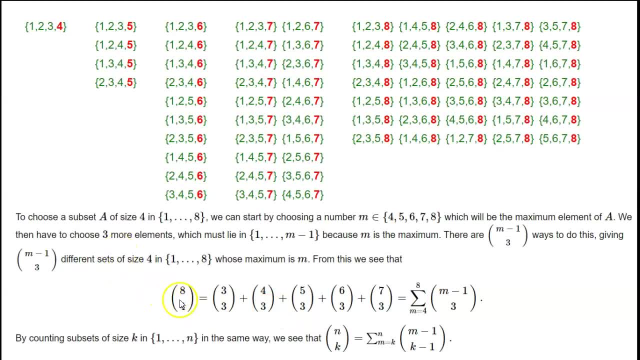 And we're going to be looking at this in the case where our n is 8 and our m is 4.. Okay, so on the left-hand side, we've got 8, choose 4.. On the right-hand side, we've got a bunch of binomial coefficients. 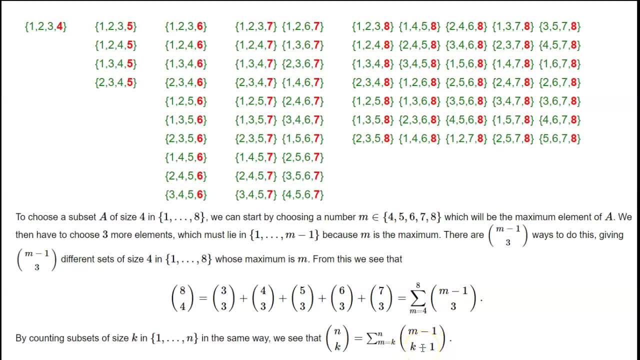 On the bottom of each binomial coefficient we have k minus 1.. Now k was 4, so k minus 1 is 3.. So we've got a bunch of binomial coefficients with 3 on the bottom, And on the top you've got m minus 1.. 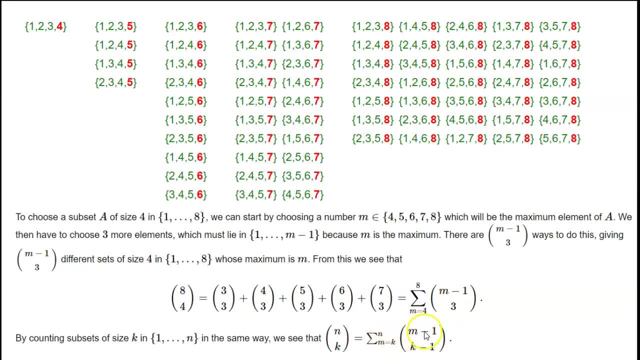 So m is running from k up to n. So m minus 1 is running from k minus 1 up to n minus 1.. k minus 1 is 3, and n minus 1 is 7.. So we've got all these binomial coefficients with a 3 on the bottom and a 3 up to 7 on the top. 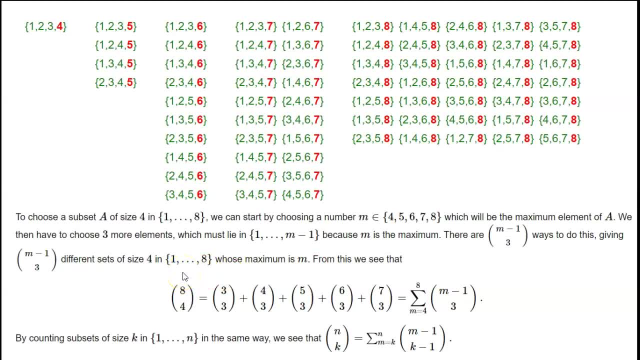 So on the left-hand side side, of course, eight choose four. that's the number of subsets of size four. uh, in in the set, one up to eight. and the idea is that we're going to break these up into five different groups of sizes: three choose three, four choose three. up to seven choose three. and the way we do this is just by splitting. 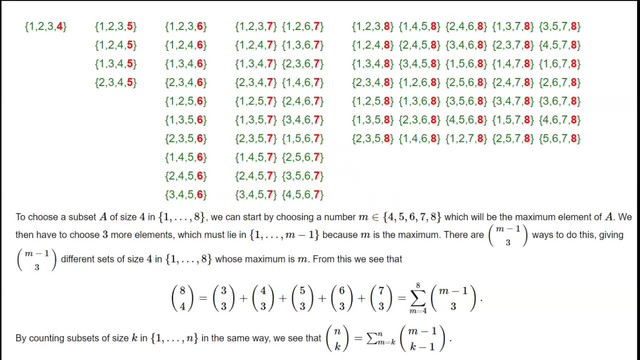 everything up according to what's the maximum element in your set. okay, so over here i mean here's a bunch of sets of uh, sets of size four in one, up to eight, and all these ones, the last element is eight, and then in all these ones here, the last element is seven. these elements of these. 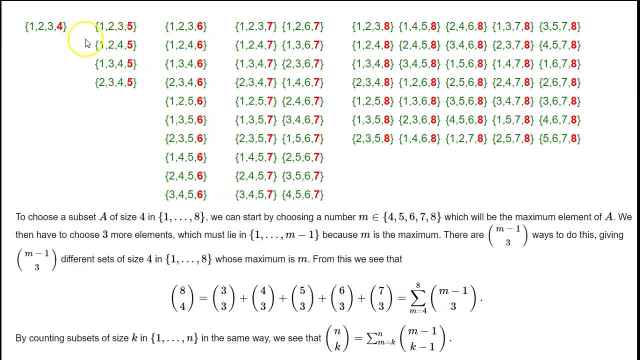 uh, sets, here the last element is six, here the last element's five, that, here the last element's four. notice: the element last element has to be at least four, because if it was less than four then you know you wouldn't have space to have four elements in the set. okay, so, uh, you know. 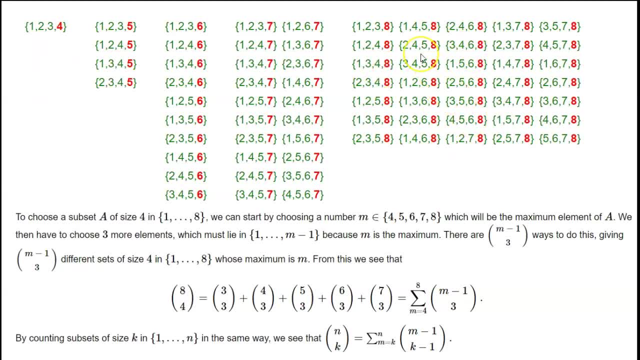 how big are these groups? right, this last group here, uh, you've got an eight and then you've got three more elements, and because eight's the last element, the, the previous elements, three elements, they have to be in the range one up to seven. okay, so the number of possibilities 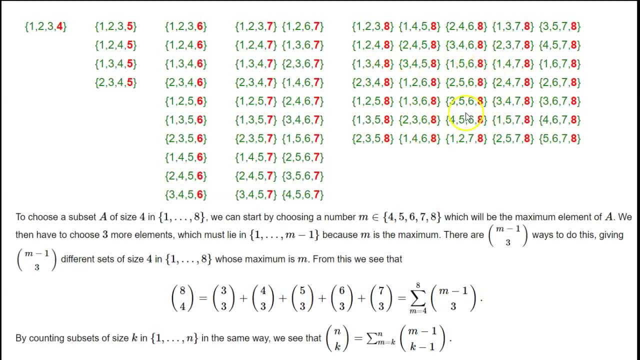 here we have the eight, and then we've got three elements chosen, from one up to seven. so there's seven. choose three possibilities which corresponds to this term here, then in this group here, these are all the ones where the last element is seven, and then you've. 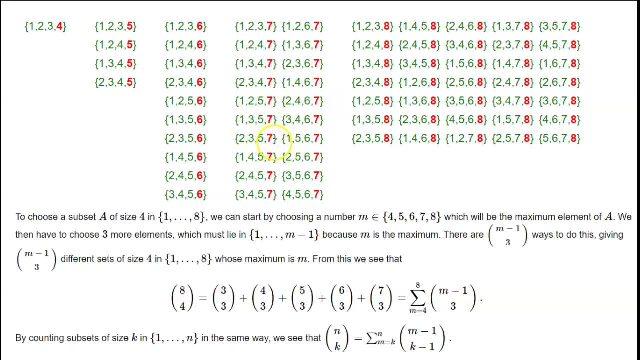 got three more elements and they have to be in the range one up to six. but you can't have the seven or the eight because you've got seven already and seven's supposed to be the largest element, so you can't have an eight. so you've got three elements taken from one up to six. 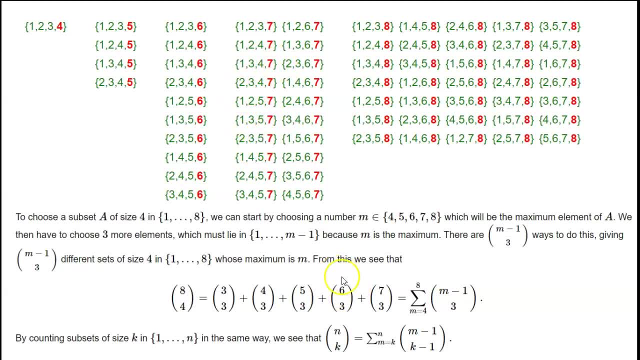 so the number of possibilities for that is going to be six. choose three. that corresponds to this term here and here. the last element is six. three more elements, from one up to five. so there's five. choose three possibilities for that. that's this, that's this term here and then here the last. 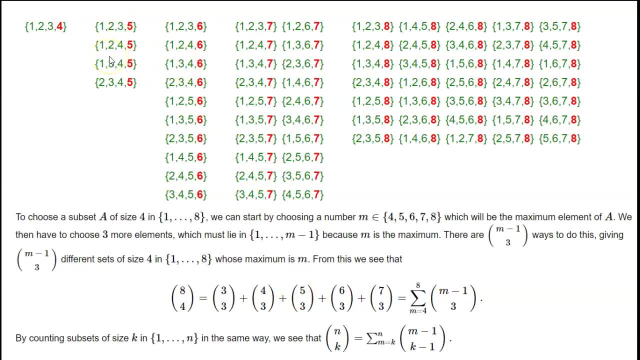 element is five, uh, three, more certain numbers that have to come from the range one up to four. so there's uh, there's uh four. choose three ways to do that, and that's this term here. and finally, the last element could be four, and then you have to have three elements taken from. 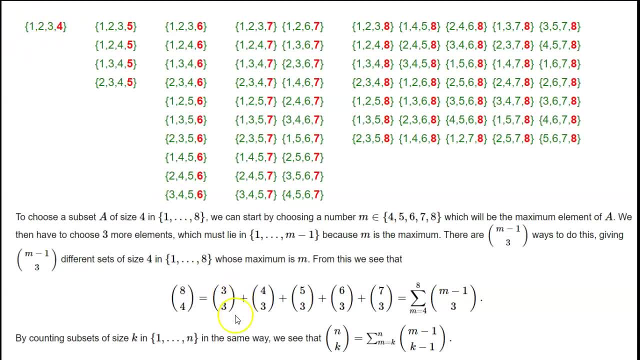 one up to three. there's only one way to do that: three choose three is one way to do that. so that's this. uh first, uh, first term here. so we've got uh eight choose four sets all together split into groups of size: three choose three, four choose three, five choose three, six choose. 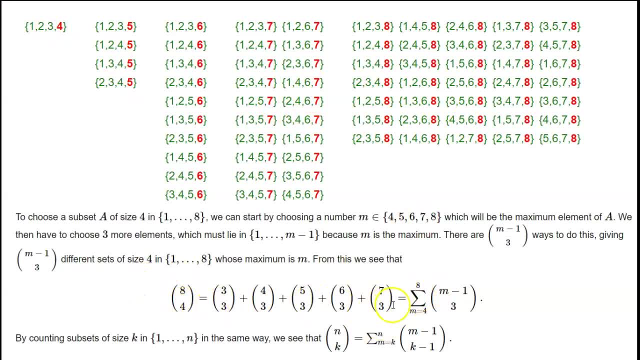 three and seven choose three. so we see that h is four is equal to the sum of these terms.